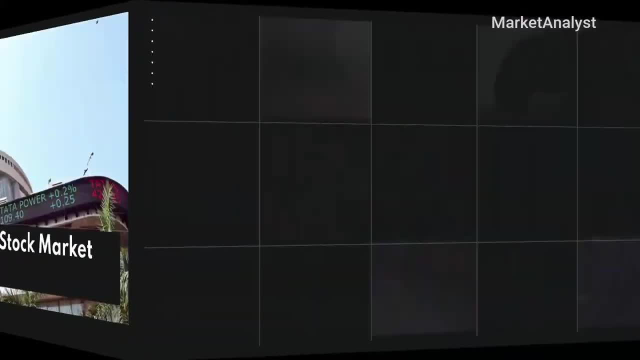 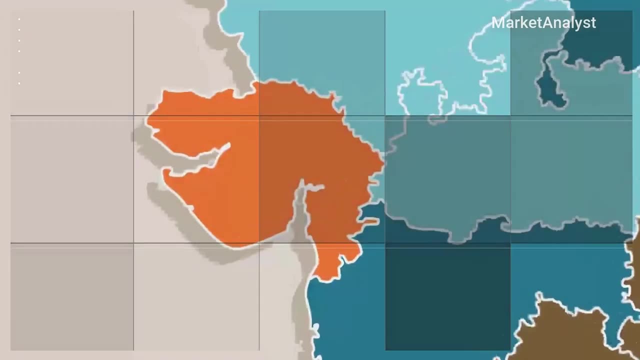 Why did the Indian stock market crash in 1992?? The stock market crash in India in 1992 was because of Harshad Chantal Almeida, an Indian stockbroker from Gujarat, in which he, along with other bankers and politicians, 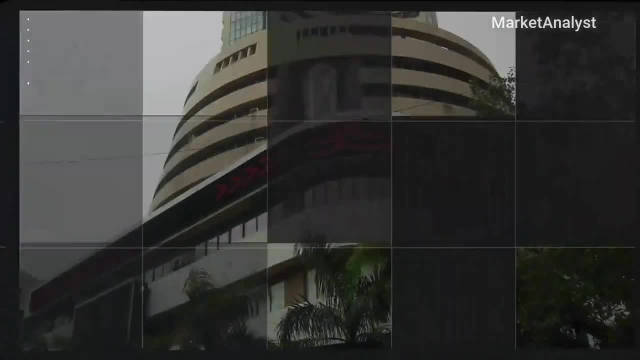 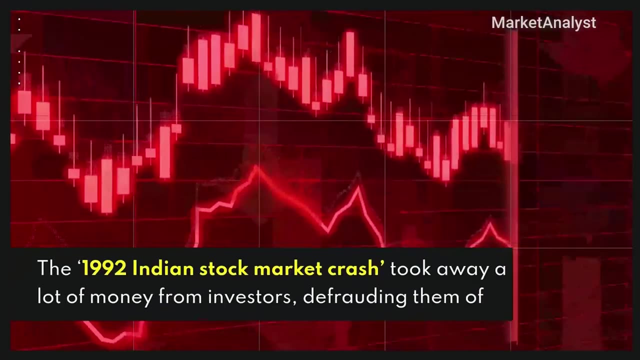 plotted a big scam against the Indian stock market. The scam toppled the Bombay Stock Exchange and caused a lot of disruption in the economy. The 1992 Indian stock market crash took away a lot of money from investors, defrauding them of over 10 million US dollars. 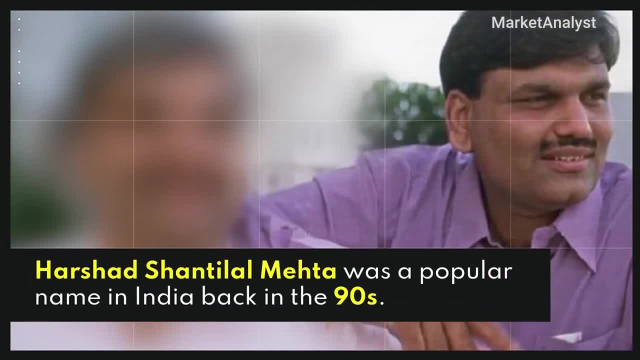 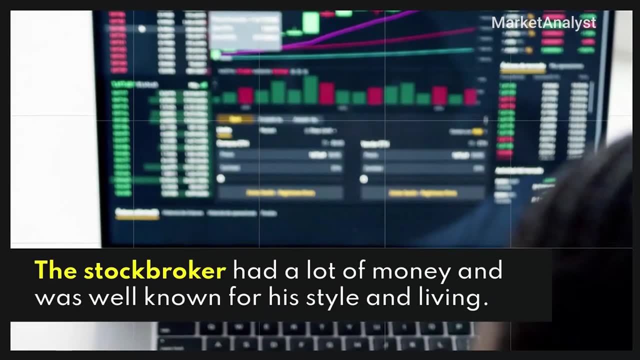 Harshad Chantal Almeida was a popular name in India back in the 90s. He was referred to as the Big Bull of the Indian stock market. The stockbroker had a lot of money and was well known for his style and living. 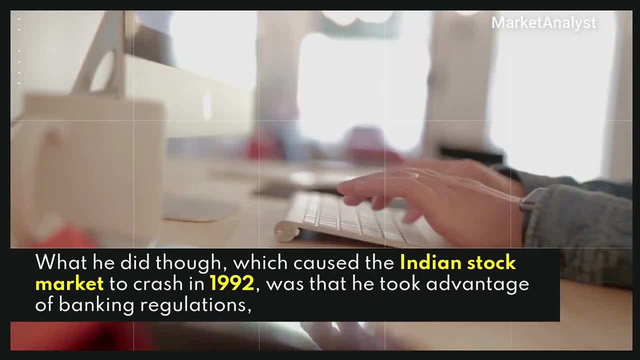 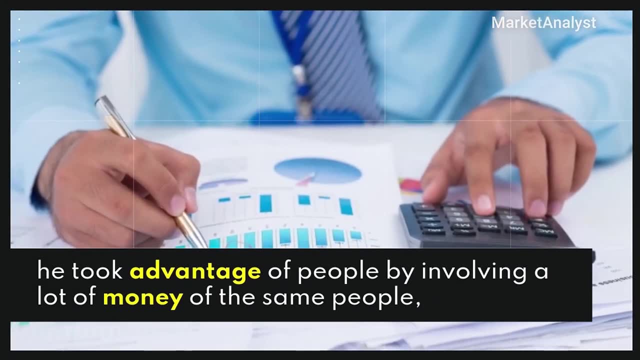 What he did, though- which caused the Indian stock market to crash in 1992, was that he took advantage of banking regulations. He took advantage of people by involving a lot of money of the same people. He used fake bank receipts and he invested in securities that were 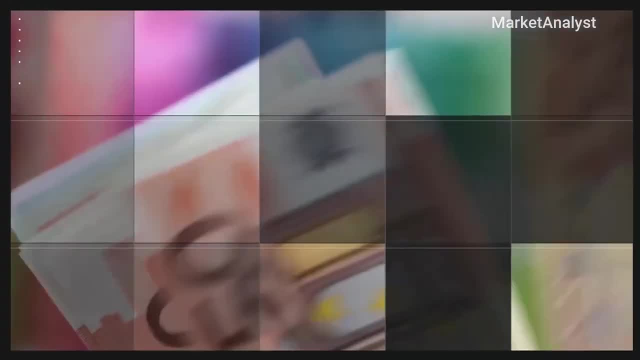 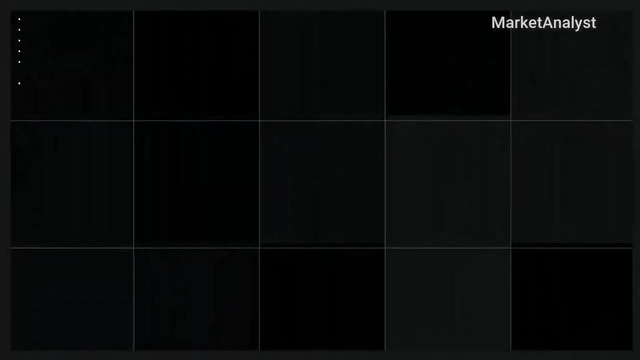 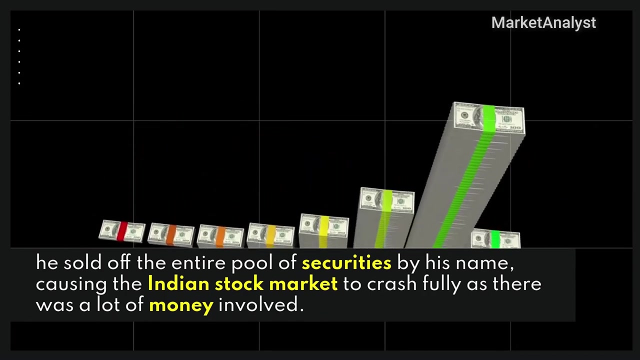 at the end of everyone's investment entirely his Inevitably one fine day. after splitting certain profits with banks and the same people who invested with him, he sold off the entire pool of securities by his name, causing the Indian stock market to crash fully, as there was a lot of money involved. Harshad Chantal Almeida was. 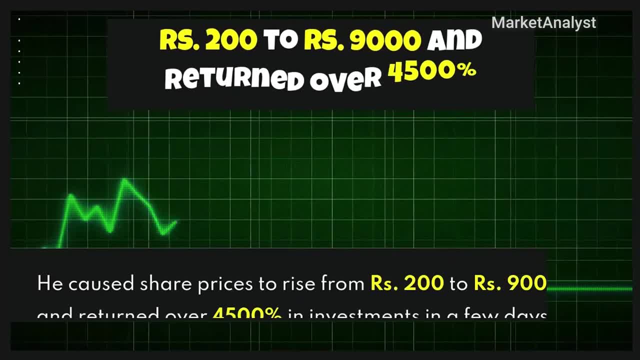 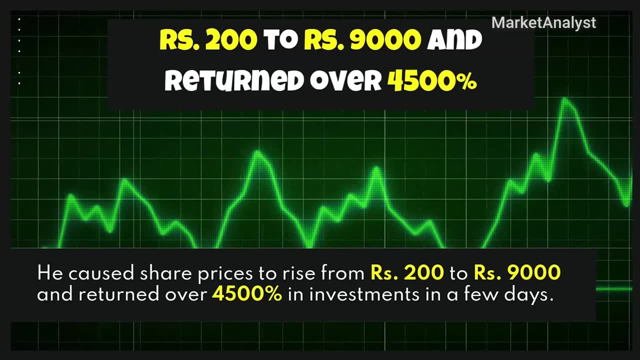 known to trade heavily. He caused share prices to rise from 200 rupees to 9.5.. He sold securities to 9,000 rupees and returned over 4,500% in investments in a few days. This appealed to bankers and they decided to invest more with him. 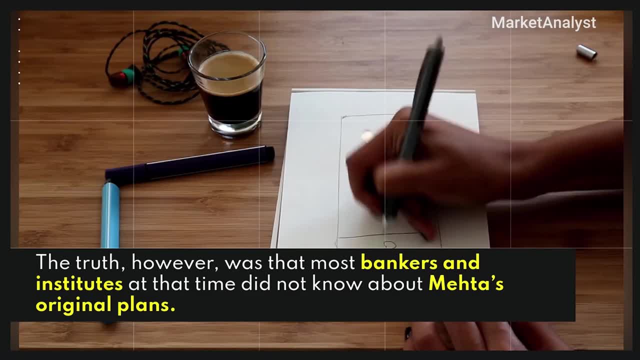 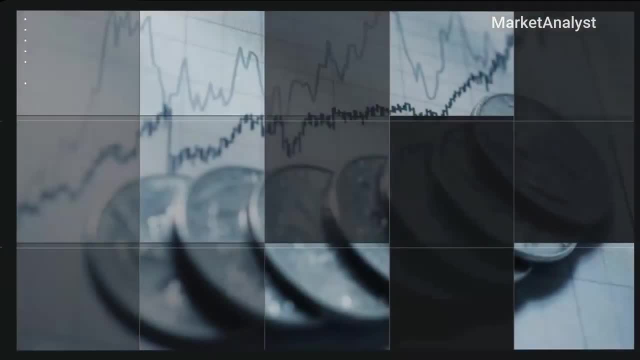 The truth, however, was that most bankers and institutes at that time did not know about Meta's original plans. He took a lot of money from his friends who were bankers at that time and fooled them by selling off all the securities even they had invested in and without their 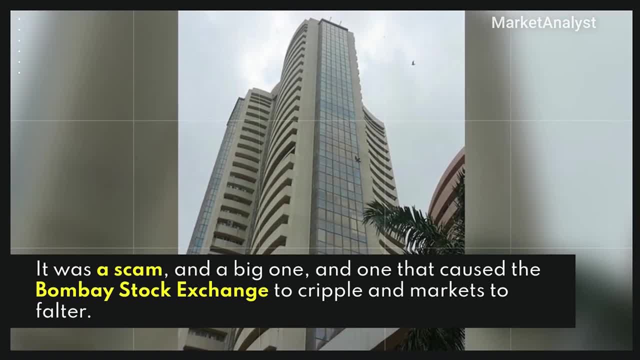 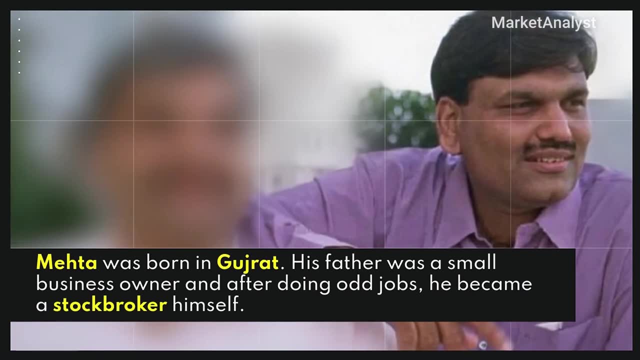 permission. It was a scam, and a big one, and one that caused the Indian stock market to crash. It was also a scam and a big one, and one that caused the Bombay Stock Exchange to cripple and markets to falter. Meta was born in Gujarat. His father was a small business owner and, after doing odd jobs, he became a stockbroker himself. Prior to the crash, Harshad became a member of the Bombay Stock Exchange as a stockbroker. Soon after he started his own firms by the name of Gromore Research and Asset Management. As a broker, he made a name for himself and invested in stock markets. 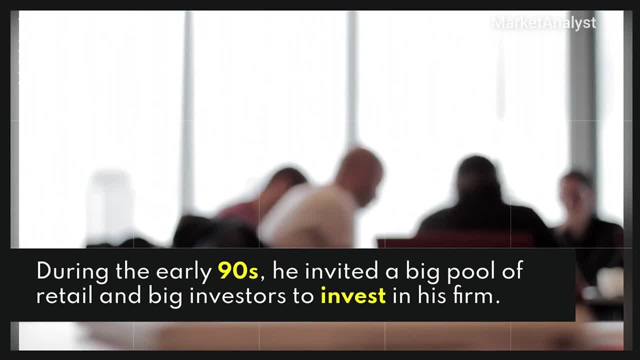 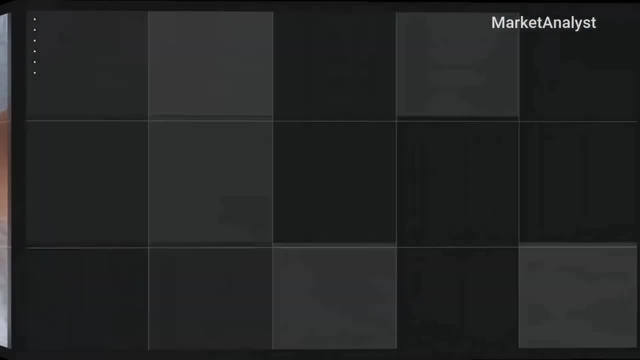 early 90s, he invited a big pool of retail and big investors to invest in his firm. Furthermore, he encouraged them to use his services to make more money. During the 90s in India, banks were not allowed to trade or invest in stock markets. Thus, a bank 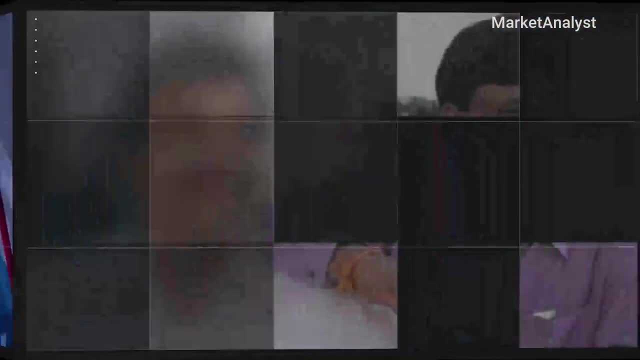 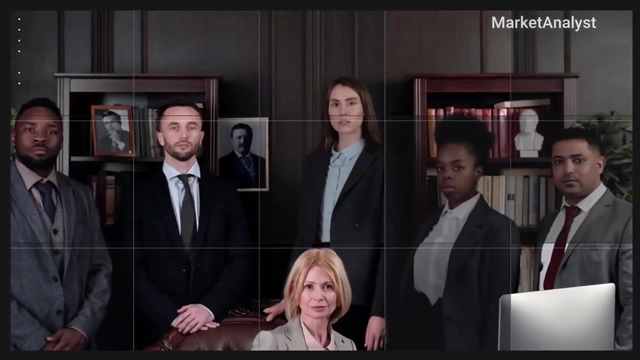 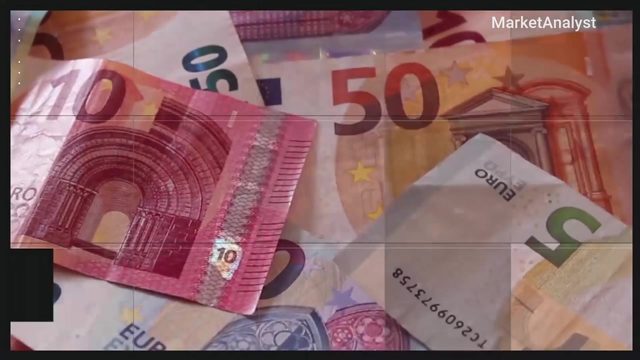 could buy stocks or bonds from a stockbroker, So they did with him. However, there was a big loophole in the system and Mehta took advantage of that. The Indian stock market crash in 1992 was around investors' trust in Mehta and how he fooled them, Essentially after the investors' 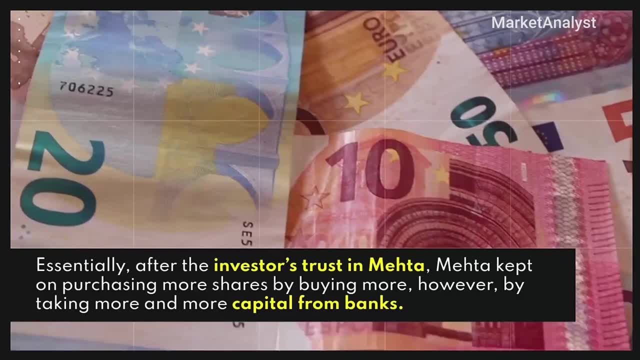 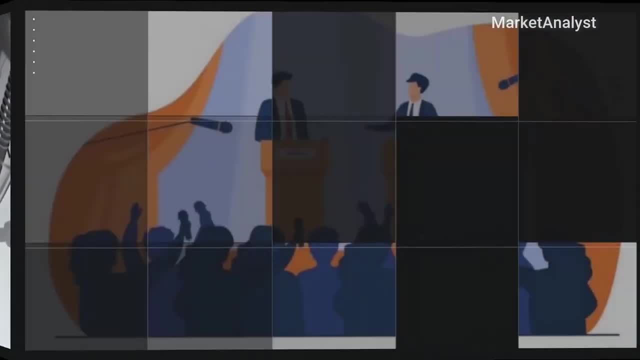 trust in Mehta. Mehta kept on purchasing more shares by buying more, however, by taking more and more capital from banks, This inevitably left them with little at the end. A lot of bankers and politicians were now involved in the scam, as they had lent him money and didn't necessarily know of. 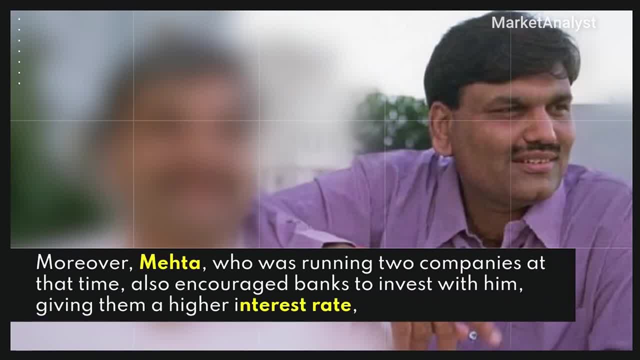 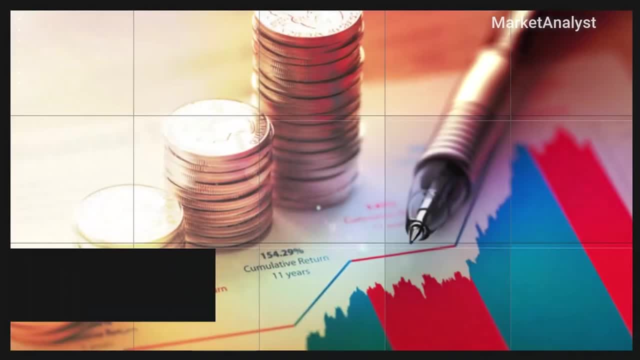 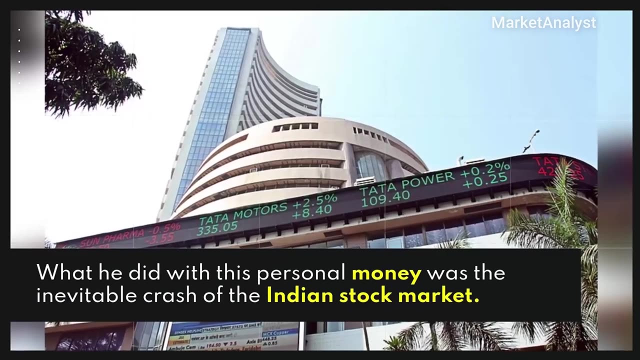 his plans. Moreover, Mehta, who was running two companies at that time, also encouraged banks to invest with him, giving them a higher interest rate, However asking the institutions to transfer the money in his personal account in return. What he did with this personal money was the inevitable crash of the Indian stock market. 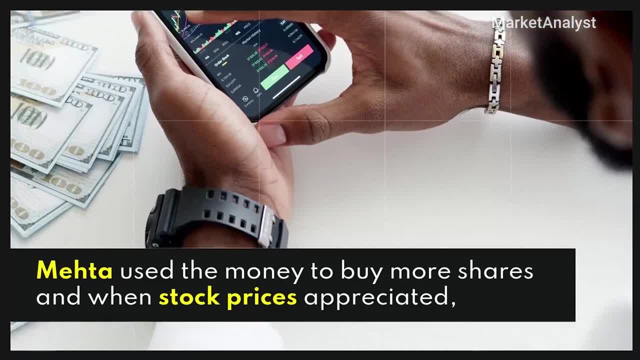 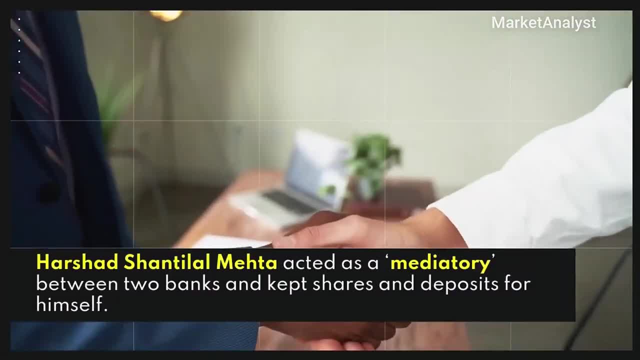 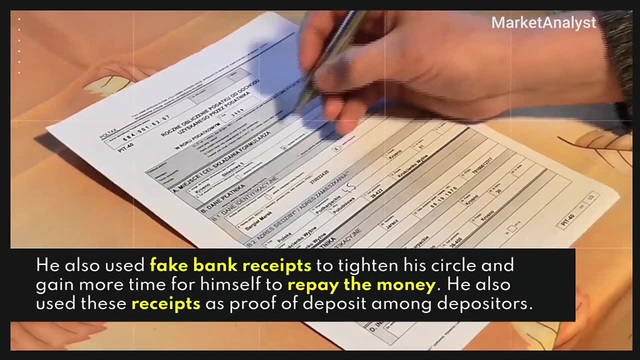 total amount for investment in the Indian stock market. Harshad Shantilal Mehta acted as a mediatory between two banks and kept shares and deposits for himself. He also used fake bank receipts to tighten his circle and gain more time for himself. 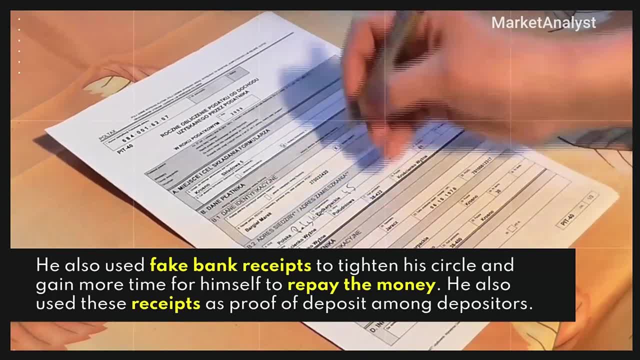 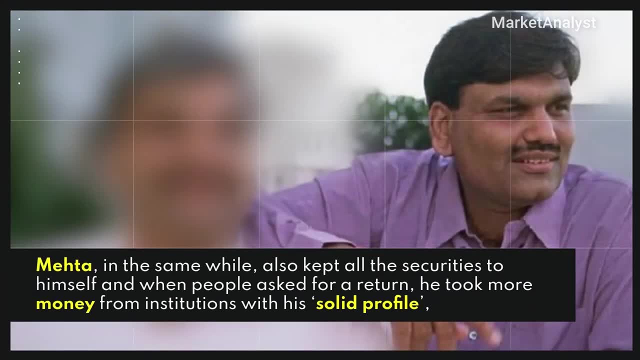 to repay the money. He also used these receipts as proof of deposit among depositors. Mehta in the same while also kept all the securities to himself, and when people asked for a return, he took more money from institutions with his solid profile And as a top investor. 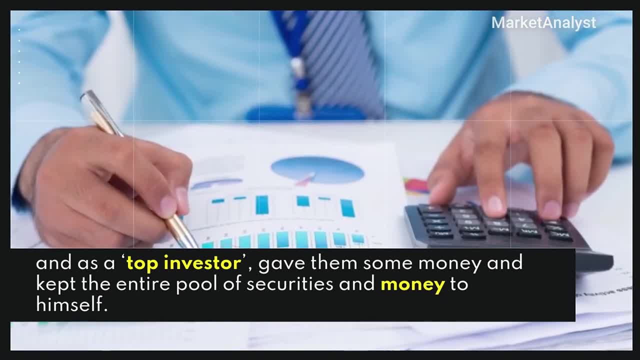 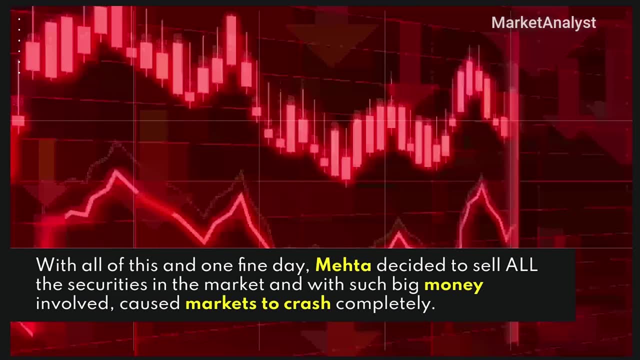 he gave them some money and kept the entire pool of securities and money to himself. With all of this, in one fine day Mehta decided to sell all the securities in the market and, with such big money involved, caused markets to crash completely.